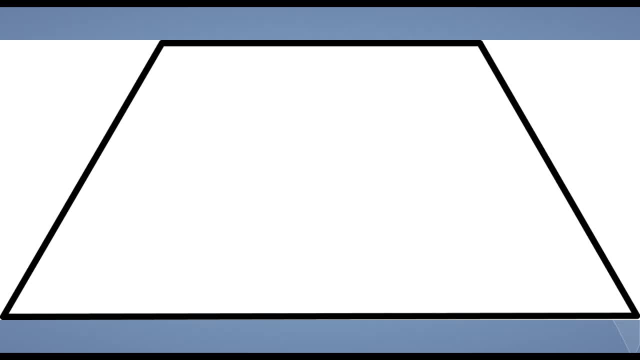 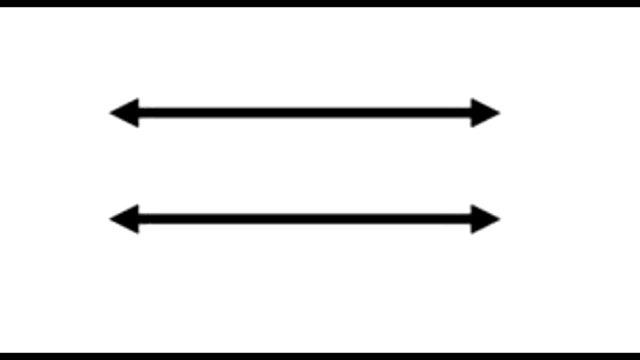 that shape is a parallelogram. If a quadrilateral has only one pair of parallel lines, or no parallel lines, it is not a parallelogram. Do you remember what parallel lines are? Parallel lines are lines that are always the same distance apart and will never meet, So in this square. 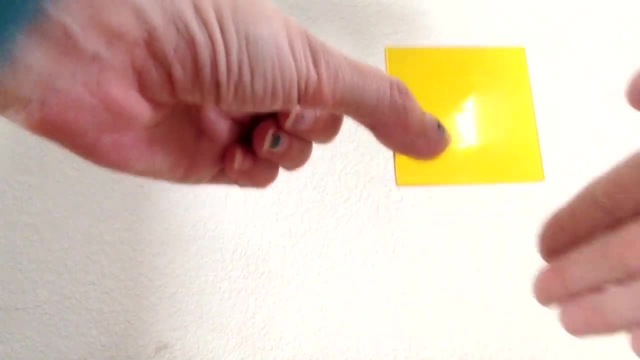 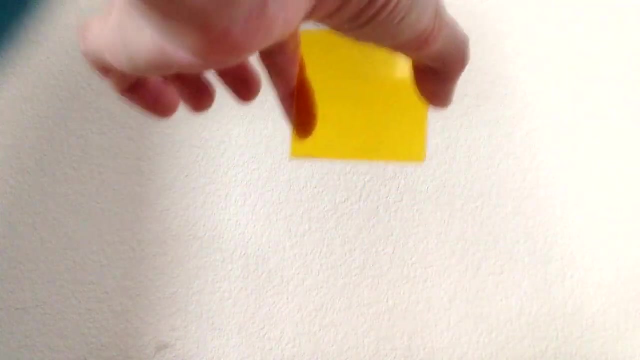 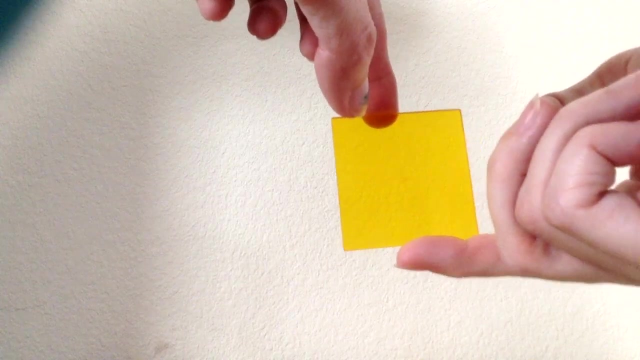 all of these lines are parallel, They're always the same distance apart and they'll never ever meet. So this has got two pairs of parallel lines, two here and two here. This square has parallel lines on these two sides and on these two sides, So this is a parallelogram. 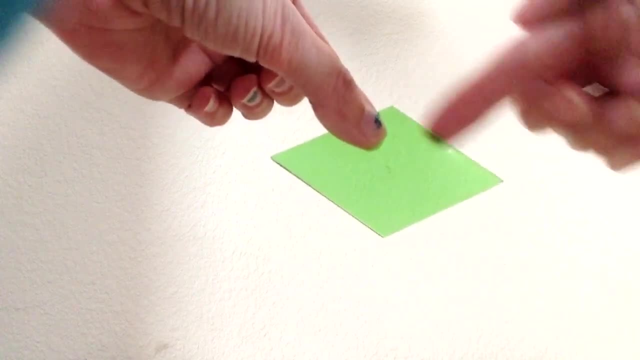 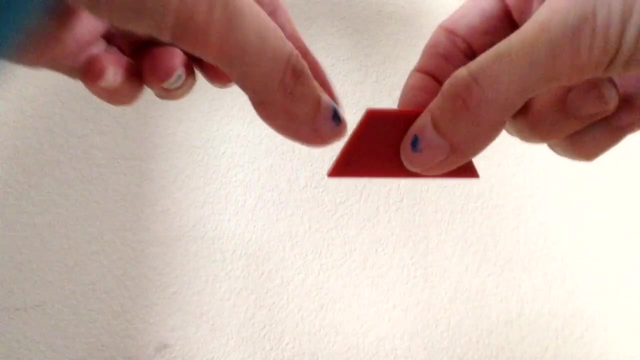 This is a parallelogram, because these lines that are opposite are parallel to each other, and these lines that are opposite are parallel to each other. This is a trapezoid. This is not a parallelogram. These top and bottom lines are parallel. 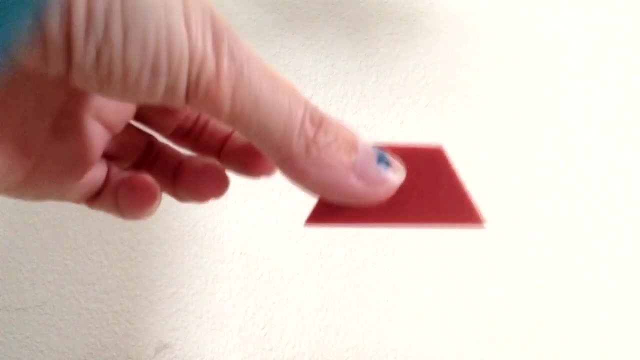 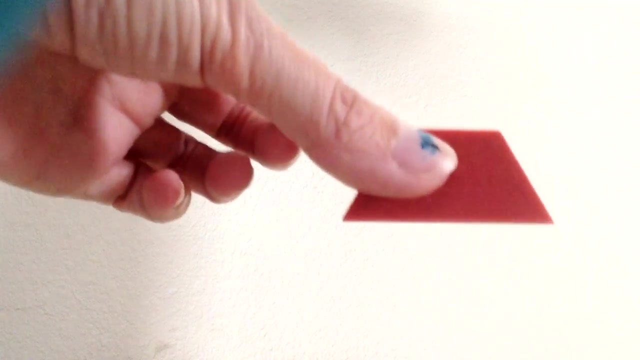 but these lines on the side are not. So let's look at some shapes. A trapezoid is a polygon because it has straight sides. It's a quadrilateral because it has four sides, but it's not a parallelogram because it has only one pair of parallel lines on the top. 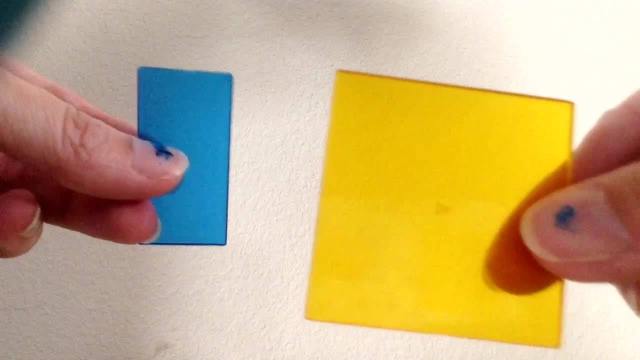 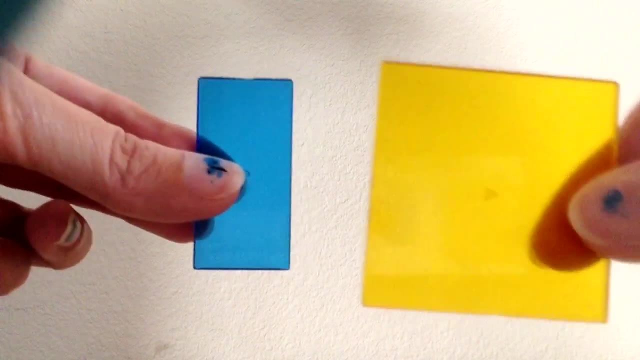 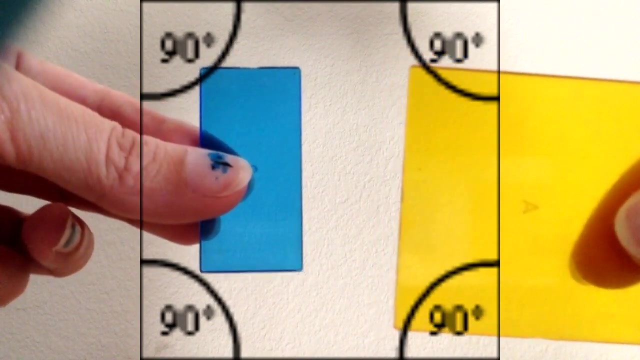 and bottom here. These are parallel. These other sides are not. And here's something else confusing: Did you know that all squares are rectangles, but not all rectangles are squares? A rectangle is a shape with four straight sides, where all interior angles are right angles. 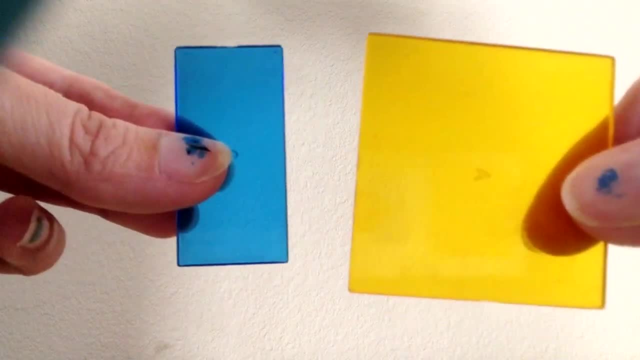 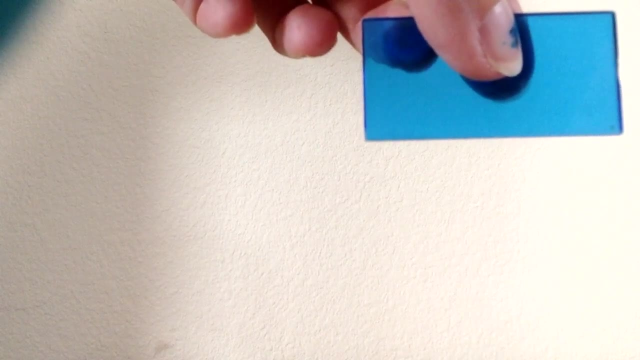 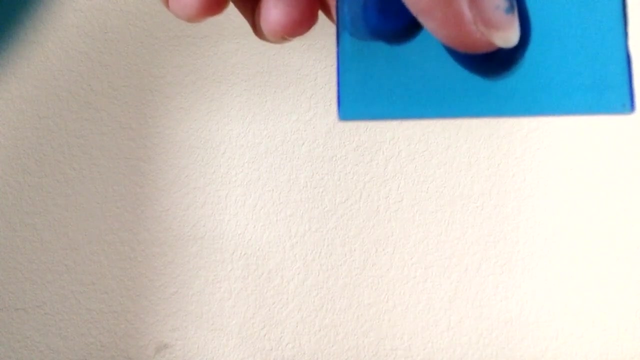 Each inside corner is a 90-degree angle. A square is a rectangle with four sides that are equal in length. Rectangles are polygons because they have straight sides, They are quadrilaterals because they have four sides And they are parallelograms because they are made up of the. 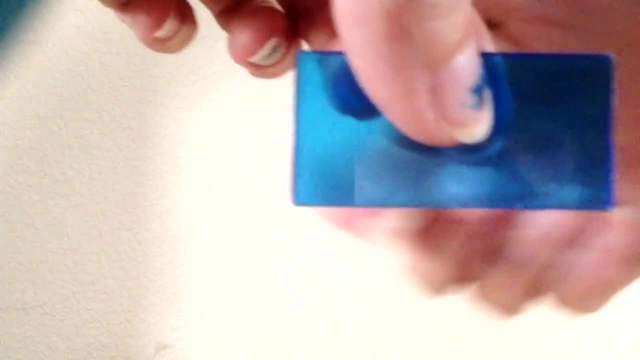 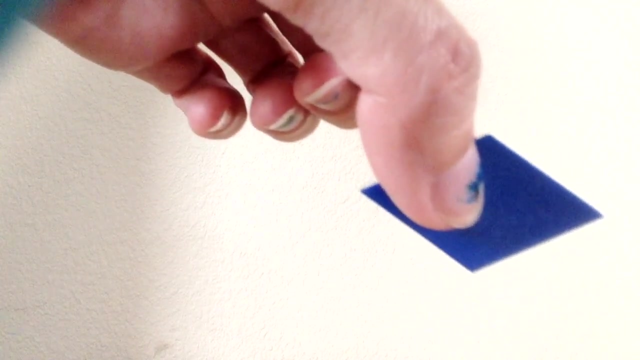 of two pairs of parallel lines. Both of these sides here on the left and right are parallel and the top and bottom lines are parallel. A rhombus is a polygon because it has straight sides. It's a quadrilateral because it has four sides.